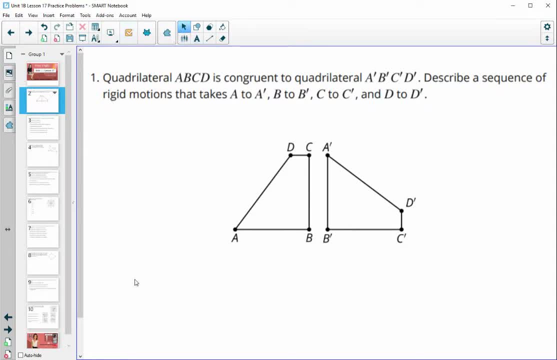 So I'm going to just type this out, But we can see that these two quadrilaterals are not touching each other, So the first thing that we're going to want to do is do a translation so that we can match up one of the vertices. 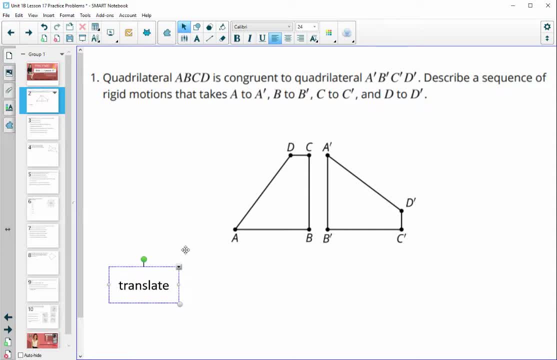 I'm just going to go with A, So translate quadrilateral A, B, C, D by directed line segment A, A, prime. This will take A onto A prime And if I just quick draw this so we can kind of see this happen. 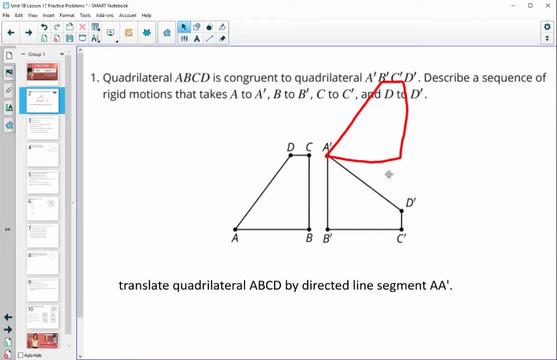 So what we've done is taken this and moved it to here And then remember that this is vertice B right here. So now what I'm going to do is I'm going to take and rotate this down so that B will land on B prime. 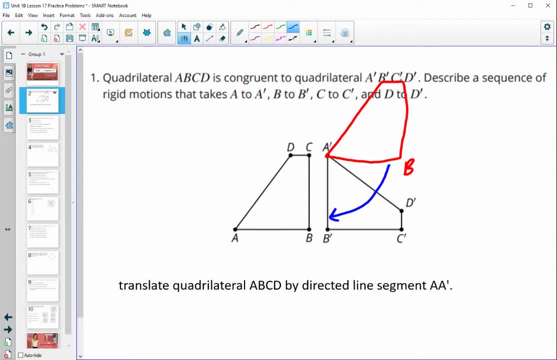 And then that's also going. We're going to at the same time take C to C prime and D to D prime, So that will be our last thing that we really need to do, And so we're going to then rotate quadrilateral A, B, C, D, using A prime as the center of rotation, until B coincides with B prime. 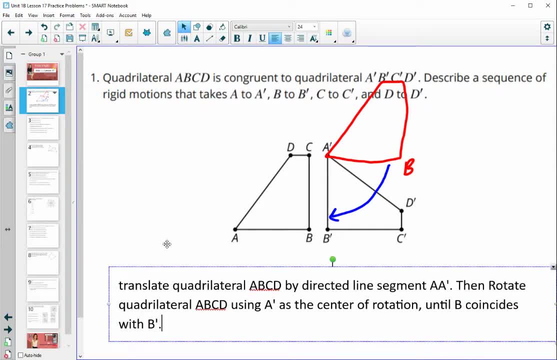 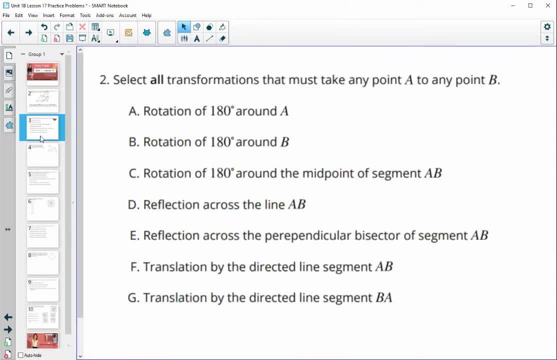 Meaning until B lands on B prime, And then everything will be matched, And that is our sequence of motions. Number two: select all transformations that must take any point A to any point B. So let me draw just any point A here and then we'll just put B here to kind of help us. 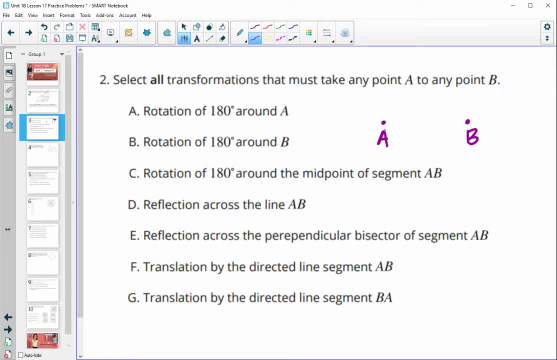 So if we were to rotate something 180 degrees around point A, would that take A to land on B? No, Okay, This is just. This is just going to be a 180 degree rotation, Not going to land it on B. 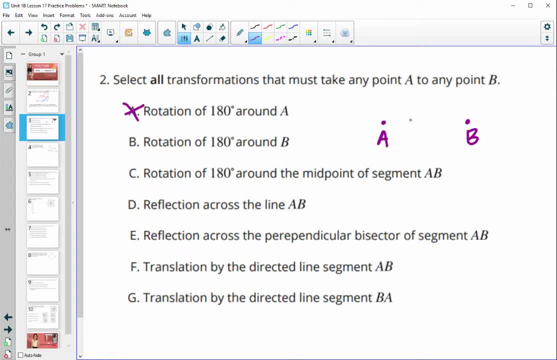 A rotation of 180 degrees around B is not going to land, It's going to land A over here, So that's going to be bad. A rotation of 180 degrees around the midpoint- So if we had the midpoint here and we just took and rotated this 180 degrees around. 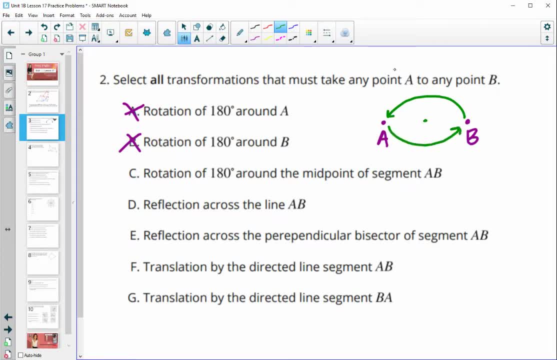 that will certainly make B Fall on A and A Fall on B, And what we're worried about is A going to B. So that will have a going to B for sure, So that one's going to be good A reflection across the line. 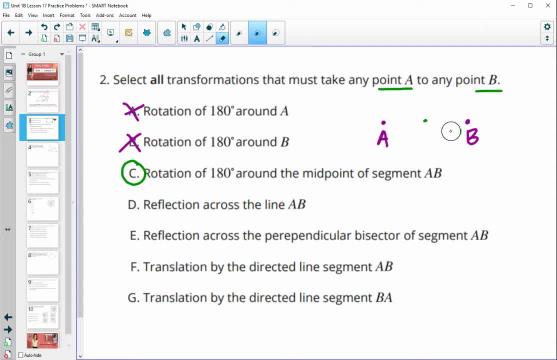 Ab Or sorry, reflection, Yeah, Reflection across the line A- B. So if we had this line here and we just reflect across the line, Is that going to flip A onto B? and that's going to be no, If we just took and rotated A to B, 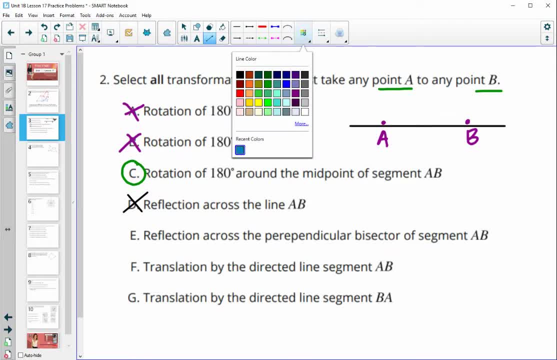 That's going to be no, If we did a reflection across the perpendicular bisector of AB, so if we had the perpendicular bisector here, that would certainly flip A onto B, So that would be good. If we do a translation by the directed line segment AB, so directed line segment AB would definitely take A over to B, because we're going to follow that direction. 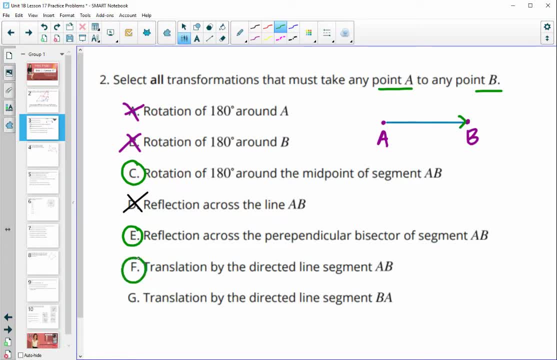 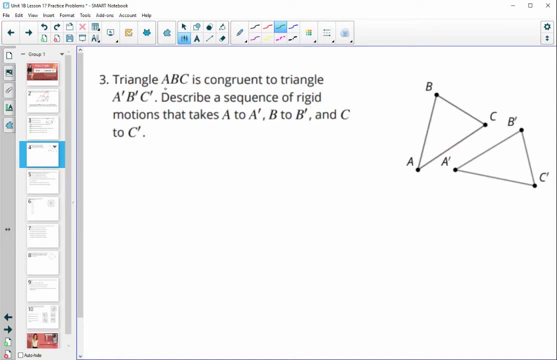 And so it's going to go this way. So this would be good, but following BA would not be good, because that would take B onto A, not A onto B. Number three: triangle ABC is congruent to triangle A, prime, B prime C prime. 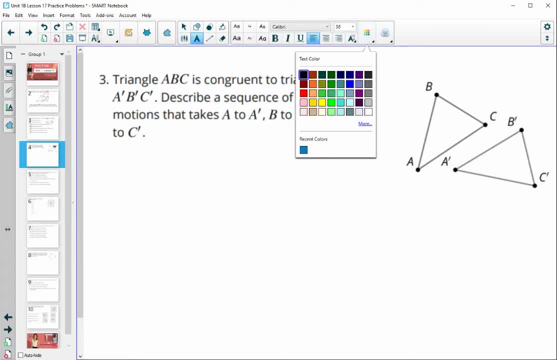 Describe a sequence of rigid motions that will take A to A prime, B to B prime and C to C prime. So again, these two triangles are not touching. So the first thing I'm going to do is do a translation. So translate triangle ABC by directed segment. 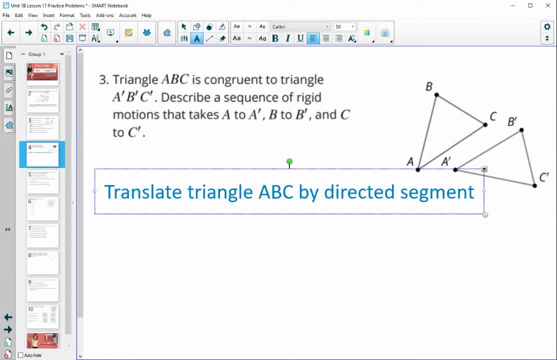 And you can choose any letters you want here. I just like to go with the first letter alphabetically. So translate triangle ABC by directed line: segment AA prime. So this is going to move A onto A prime And then we're just going to need to rotate so that B goes to B prime. 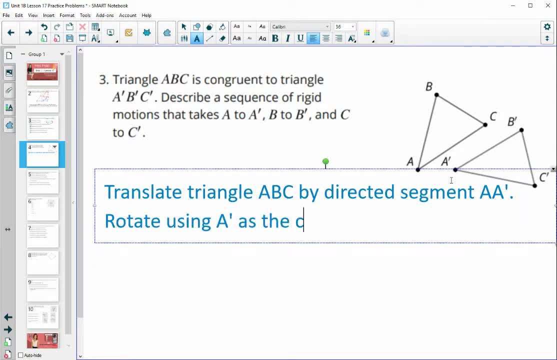 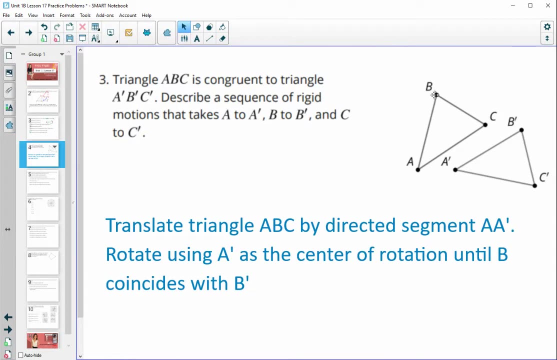 So then, rotate, Using A prime as the center of rotation, until B coincides with B prime. And then, since we know that the triangles are congruent, that will actually, once B hits B prime, that will force C to land on C prime as well. 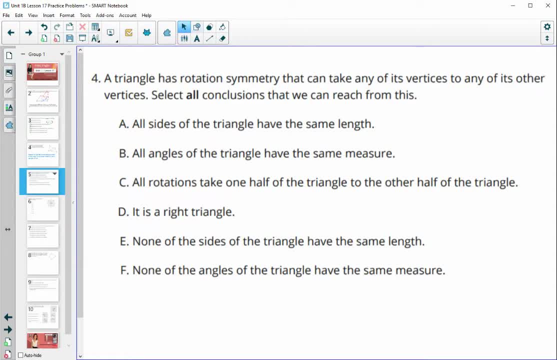 Number four: a triangle has rotational symmetry that can take any of its vertices. So this is going to be a triangle that can take any of its vertices to any of the other vertices- Whoops. So all the vertices can be taken to each other. 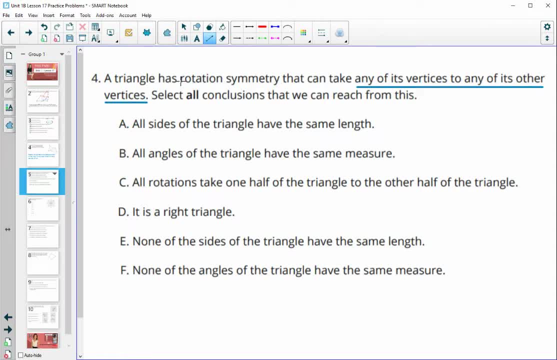 Select all of the conclusions that we can reach from this. So rotation, So every vertex is able to rotate onto any other vertex. That is going to mean that this triangle, all the sides are going to need to be the same and all the angles are going to need to be the same. 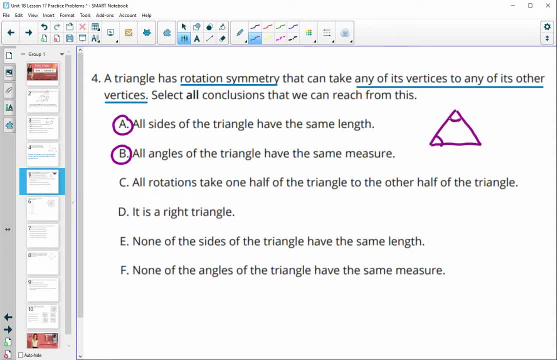 So it's going to need to be equilateral, An equiangular, so that as it rotates, OK, it'll land perfectly on either side. So when this vertex goes to here, those angles are the same And also then this side length is going to rotate to this side. would need to be the same all the way around. 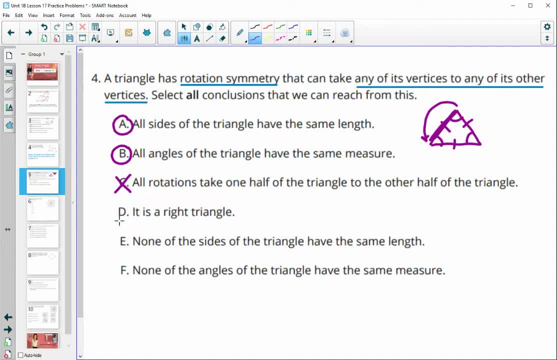 So it's not going to take half of itself onto the other half. It's not going to be a right triangle, because a right triangle would not have all of the angles be the same measure, because you'd have one 90 degree angle, And in order for them to all be the same, you need to have every angle be 60 degrees. 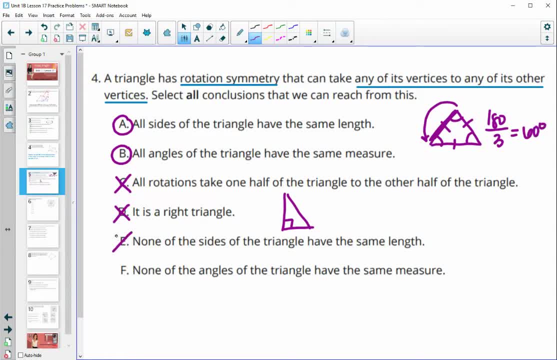 So that would not work. None of the sides have the same length- Not going to be good because they're going to have to land on each other. So they're all going to have to be the same, And then none of the angles. 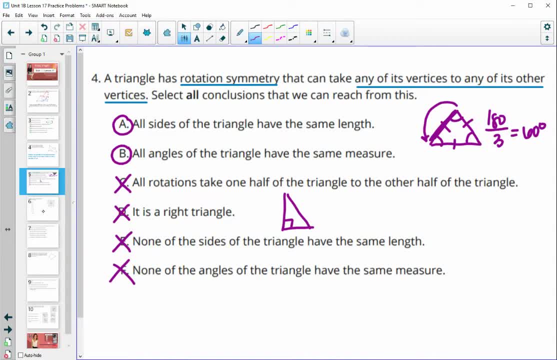 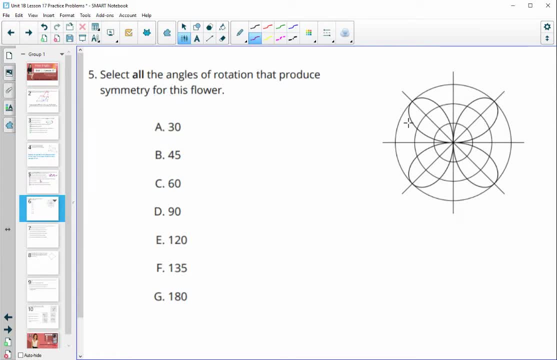 We know that's not true because they all need to be the same. All right. Number five select all angles of rotation that produce symmetry for this flower. So when we look, we kind of see four different sections that are Identical. so we're going to take 360 divided by four and that's going to give us 90 degree rotational symmetry. 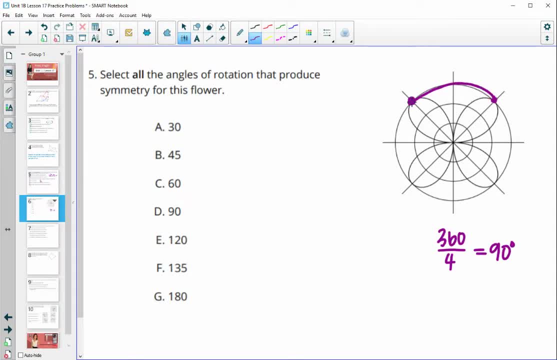 So if we take this and we rotate it, 90 degrees, it'll land here. 180 degrees, it'll land here. 270 degrees it'll land here, and then, of course, 360 will get you back to the original. 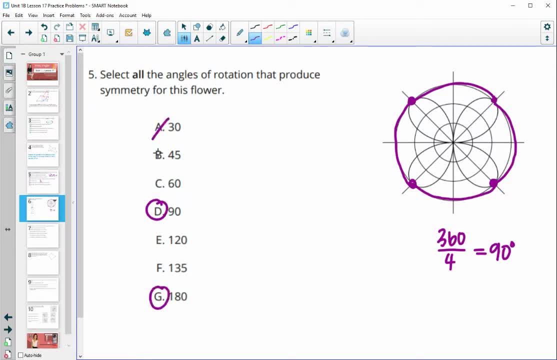 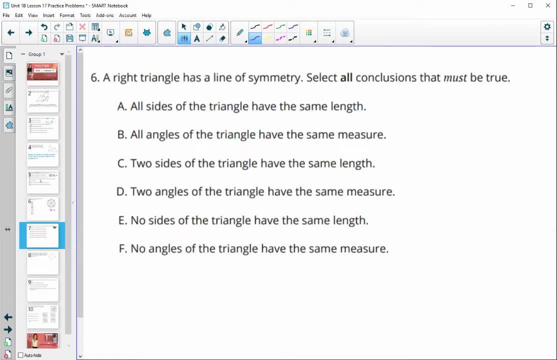 So 90 is going to work and 180 is going to work, But all these other ones are not. Number six: a right triangle has a line of symmetry. Select all conclusions. So just one line of symmetry. So all the sides of the right triangle are the same? would not be true, because then we would have three lines of symmetry. 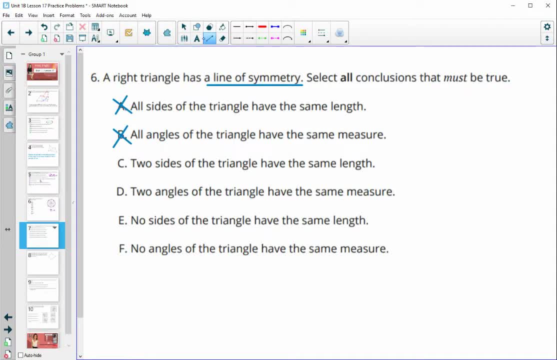 And same for the angles all being the same. So that would be an equilateral equiangular triangle. And if I draw one of those out so that you can kind of see that, So if it was like this, we would end up with more than one. 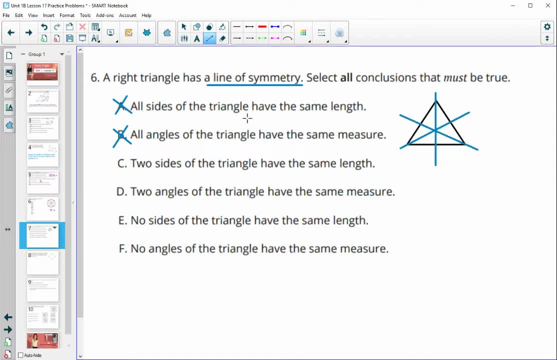 And because you'd be able to go here, here and here. So that's not going to work out. Two sides of the triangle have the same length in order to get a line of reflection. That would be fine, because then we can go between these two equal sides. 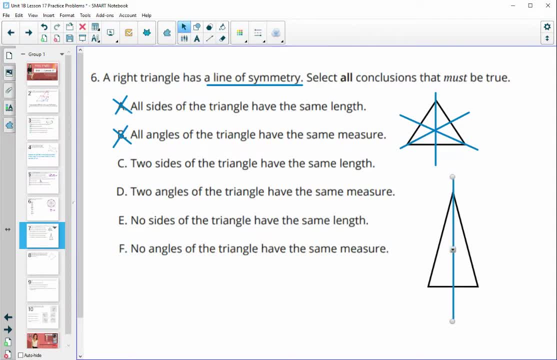 And that would produce one line of symmetry, and we won't have a line of symmetry through either of the other vertices, So that one is true. So then, two angles have the side length as same length, Same Same measure as well. So these two angles are the same in order for them to land on each other. 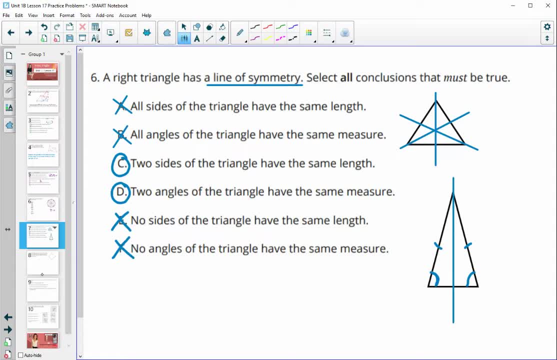 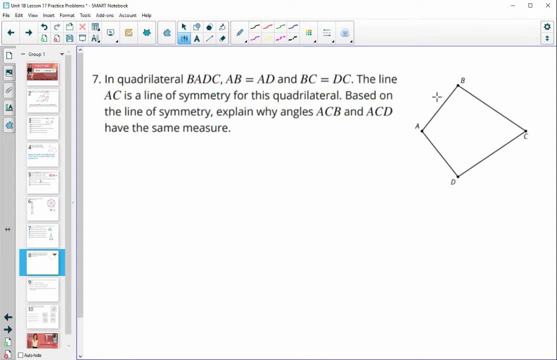 That would be true. So we know that it can't be that there's no sides or no angles, Because then nothing would flip on top of each other and be the same for symmetry, Number seven and quadrilateral BADC, AB is congruent to AD and BC is congruent to DC. 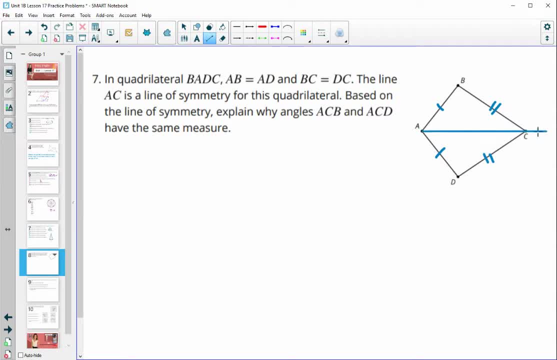 AC is a line. It's a line of symmetry. Based on the line of symmetry, explain why the two angles: A, B, C. So why is this angle and this angle? why do those angles have the same measure? So we know that point A and C will stay set in place, since they are on the line of symmetry. 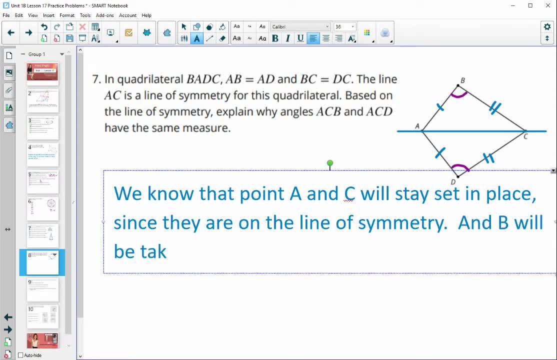 And B will be taken on to point D. So this means that with those being set and then a reflection taking it on to the other, this means that Whoops, Oops, Angle ABC has to be the same measure as A, B, C. 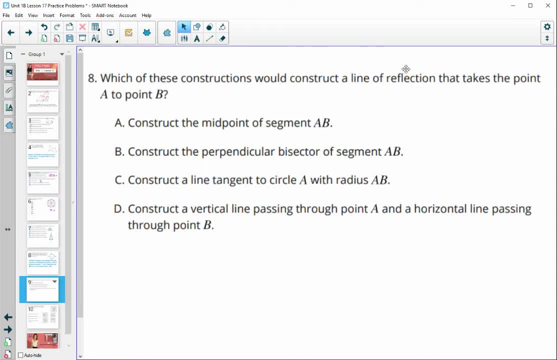 Number eight. which of these constructions would construct a line of reflection that takes point A on to point B? So we need a line of reflection, And so just constructing the midpoint won't give us a line of reflection If we construct the perpendicular bisector. 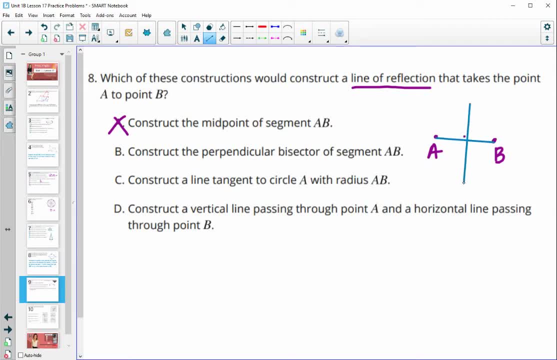 So if we connected that segment and then did the perpendicular bisector, That would certainly do it. Construct a line tangent to circle A- We don't care about that. Construct a vertical line passing through A and a horizontal line passing through B. So that would look like this: 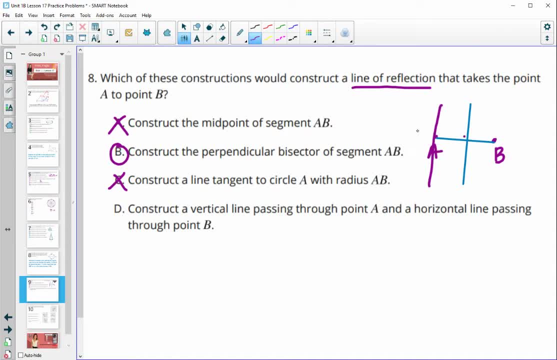 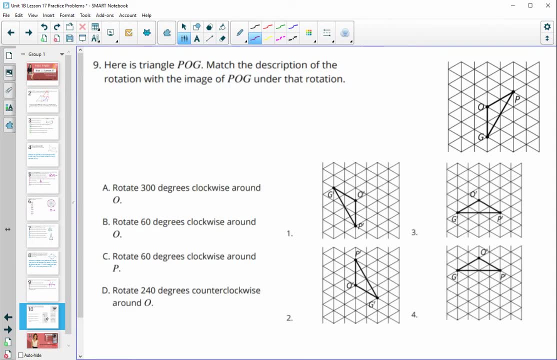 Vertical through A, Horizontal, Oops, Horizontal through B, Something like this. That's not going to do it, So B would be the answer there. And then finally, number nine. Here's triangle, POG. Match the description Of the rotation with the image of POG under rotation. 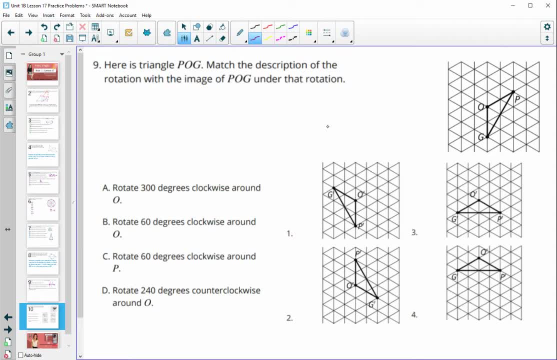 So remember that a rotation needs a center of rotation, So a point that's going to stay the same. So I'm going to look in each of these and determine what that is, Because we see that it's O in three of them and P in one of them. 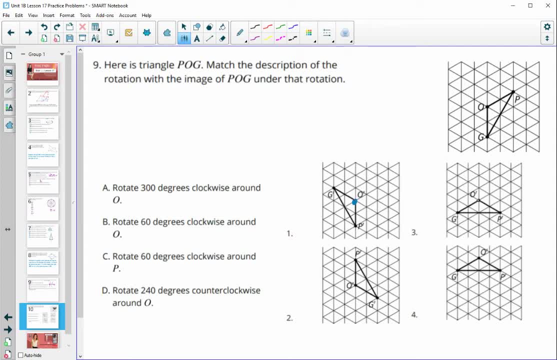 So when we look here, O prime is in the same spot. O prime is in the same spot in number three. O prime is in the same spot in number two. P is in the same spot in number four. So letter C goes with number four without question, because it's the only one that kept P in the same spot. 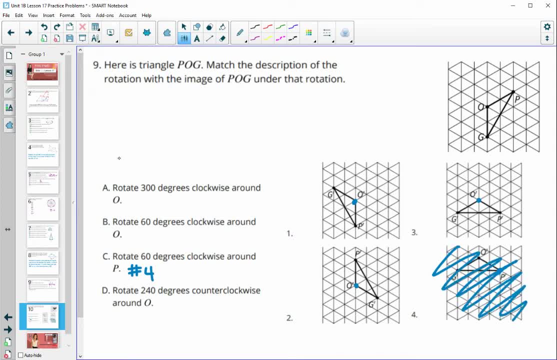 So I'm just going to cross that off so we don't have to look at it anymore. Then you want to determine how much of a rotation it is. So decide if you want to compare point G to G prime or P to P prime. 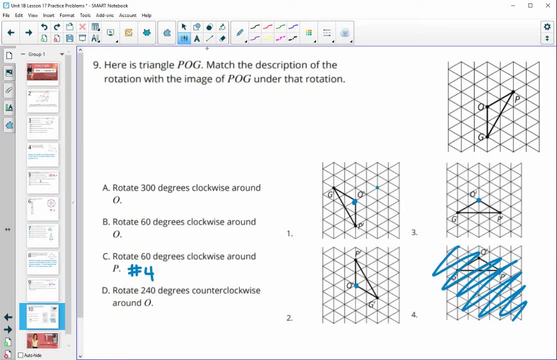 I'm going to do P, So I'm just going to draw P on here and then look at this angle. So here's where P would have been. So here's where P would have been. So here's where P would have been.